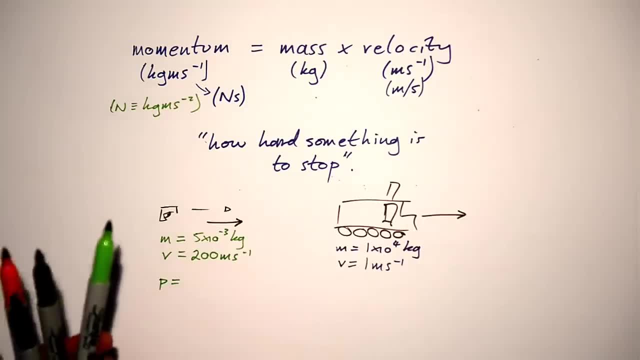 Generally little p, because big P is used more for pressure. So what do we have? Five times ten to the minus three times 200, and that gives us immediately one newton second of momentum or kilogram meters per second. I'm just going to use newton seconds. 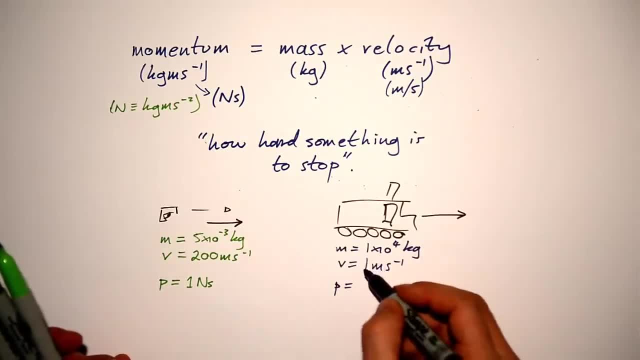 save me my sharpie ink. On the other hand, we have one meters per second, times one times ten to the four, So that's actually one times ten to the four newton seconds. So that's a lot of momentum that the train has. So, even though the bullet is traveling, 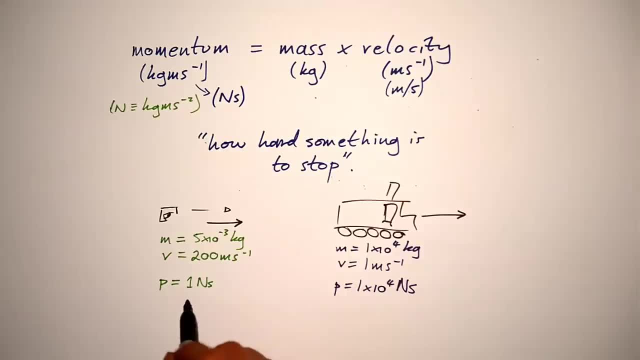 so much faster, 200 times faster. it has a tiny momentum compared to the train that's just trundling along. Which one's going to send you flying more? The train definitely will If both of these things transferred all of their momentum to you. in other words, they both stopped. 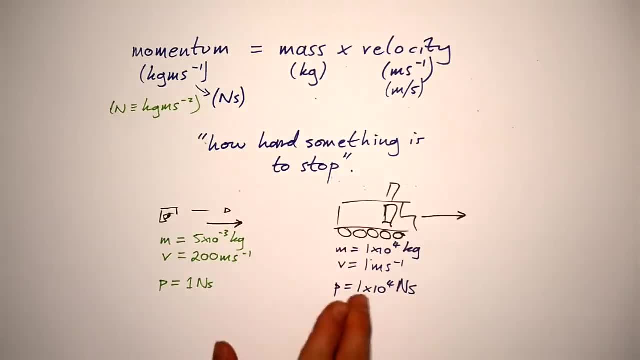 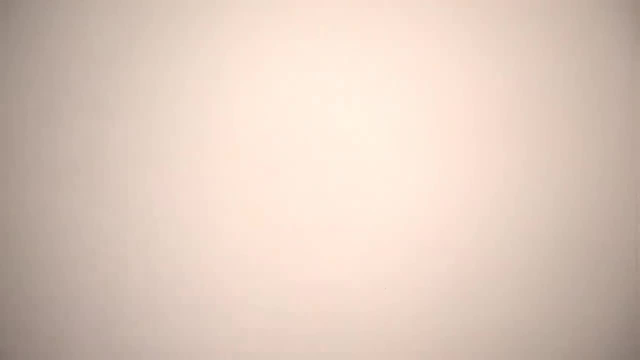 when they hit you, the bullet might send you flying a little bit. The train is going to send you absolutely flying for miles because it's got a lot more momentum to give you Now. when things collide in any way, shape or form, momentum is always conserved. 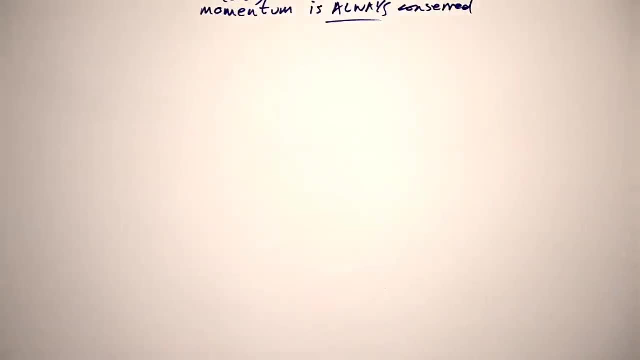 Now we should probably say that total momentum is always conserved. In other words, if you take the momentum of one thing and another thing that are crashing into each other, the total momentum of both of those things, or all of those things, is always going to be. 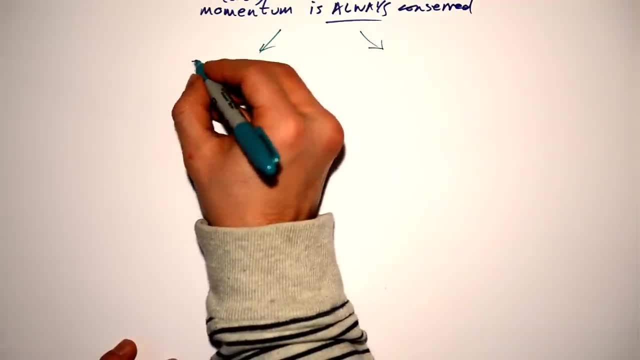 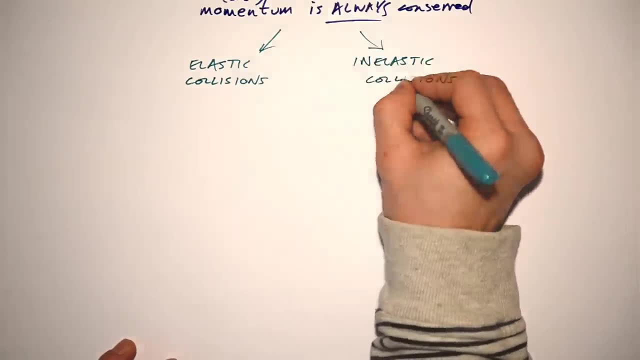 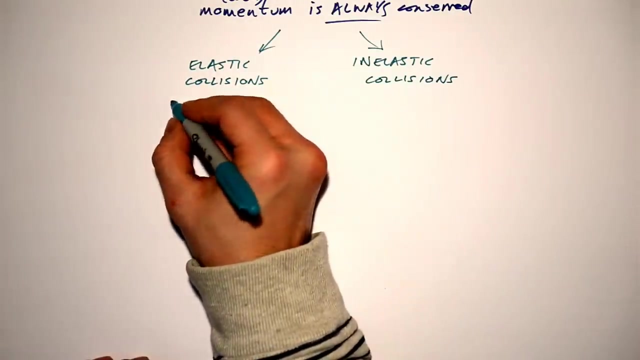 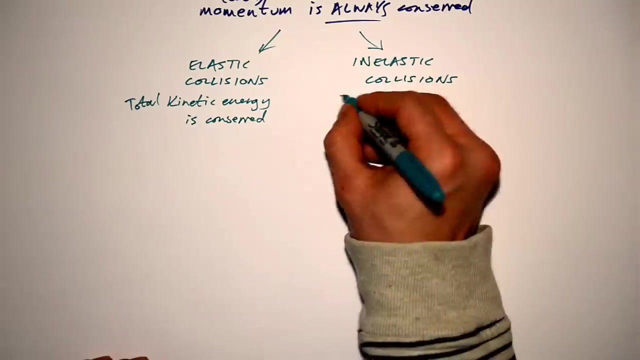 the same. Now there are two types of collisions. We have elastic collisions and we have shock-horror inelastic collisions. The only difference between these two: momentum is always conserved in both of these things. but in elastic collisions, total kinetic energy is conserved and in inelastic collisions, total kinetic energy. 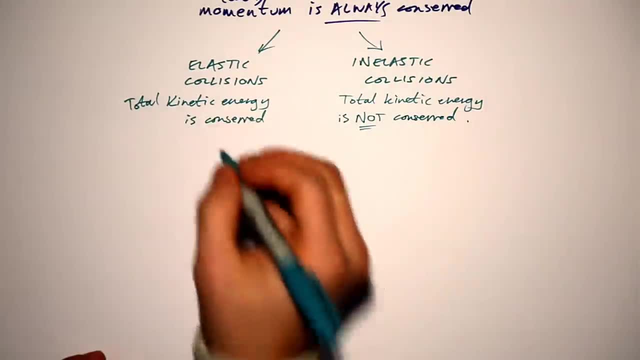 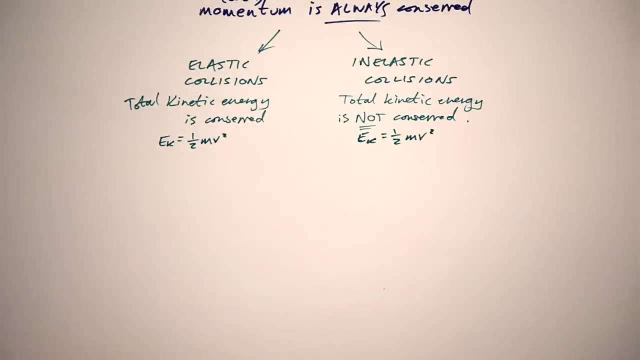 you guessed, it is not conserved, So don't forget that kinetic energy is half mv squared. I'm just going to write it as ek could get asked. Here's a collision: Calculate what's going on with the speeds and check if. 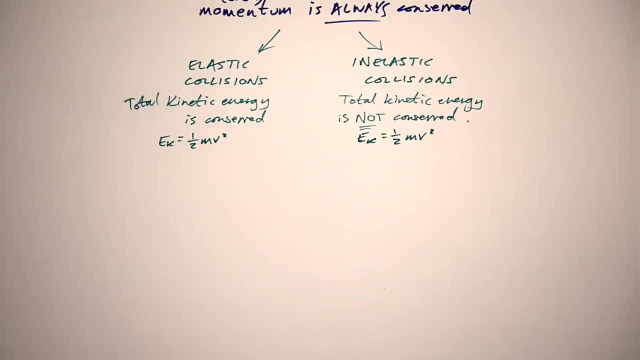 it's elastic or inelastic. So let's have a look at an example of a collision then, shall we? Let's go with coupling. This could be two train cars coupling together. One has momentum before, the other, one has momentum before and then afterwards they have the same momentum added up. 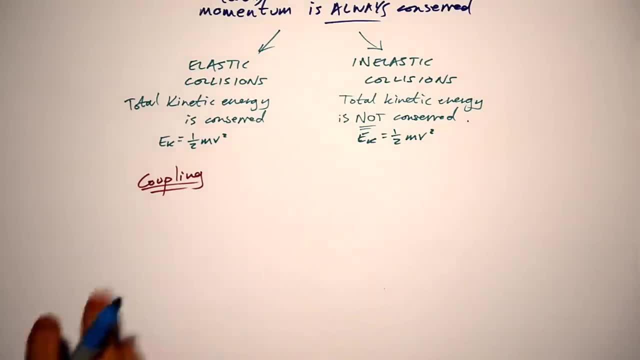 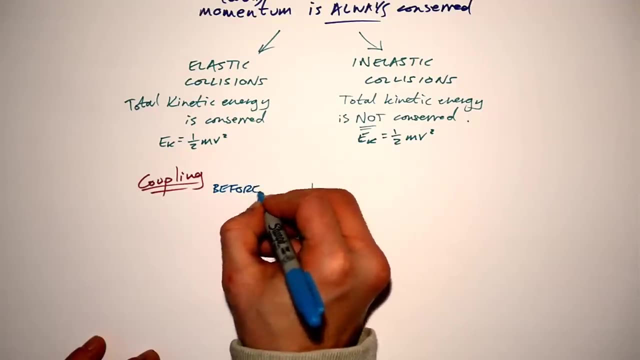 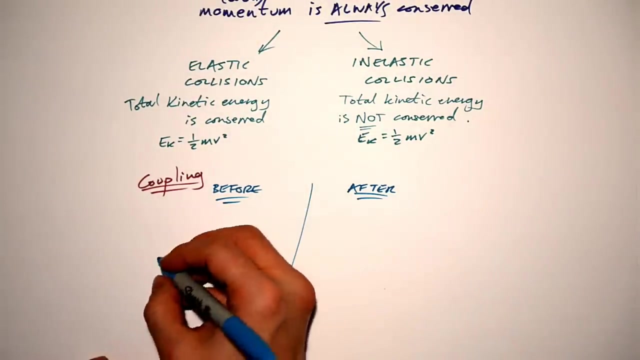 But seeing that we're talking about coupling and couples, let's go with a couple of figure skating. Now what I do is split my page in half before and after the collision. Before, what we have is the girl skating towards the guy and he's ready to catch her and he's going to lift her and they're going to go off together like so. 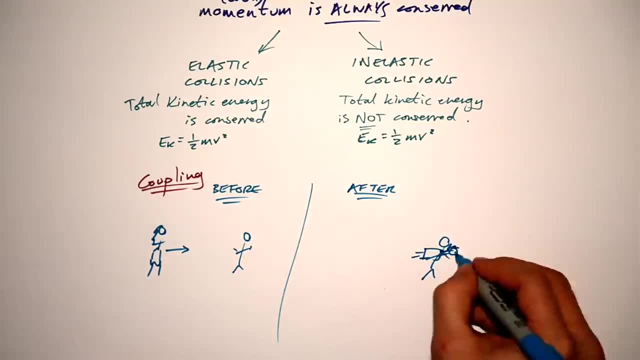 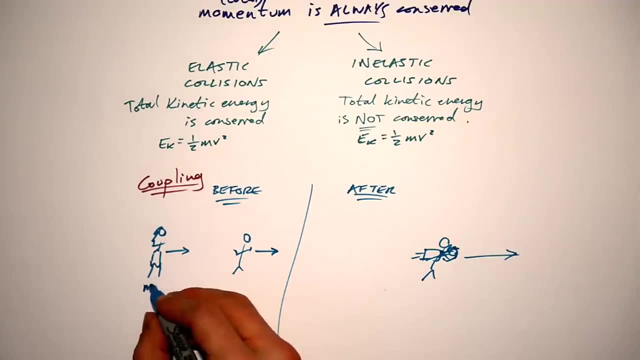 So there they are. afterwards, Let's say that the guy is also going that way as well. to begin with, We're going to call this girl m1, and she has a mass of 60 kilograms. The guy m2, has a mass of 80 kilograms. 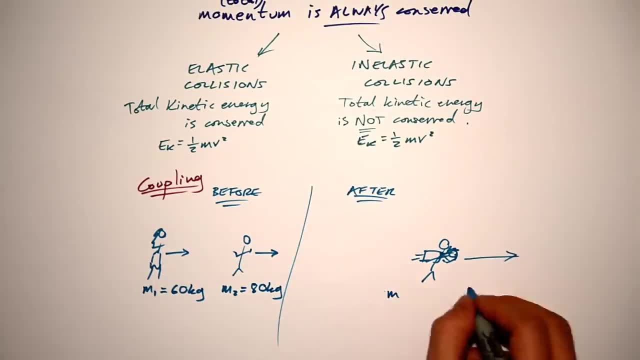 What do we know about afterwards? The mass of both of these put together. so I'm going to put m12, not m12,, but m3, m2, that's going to be equals to 140 kilograms, because they've now coupled together. 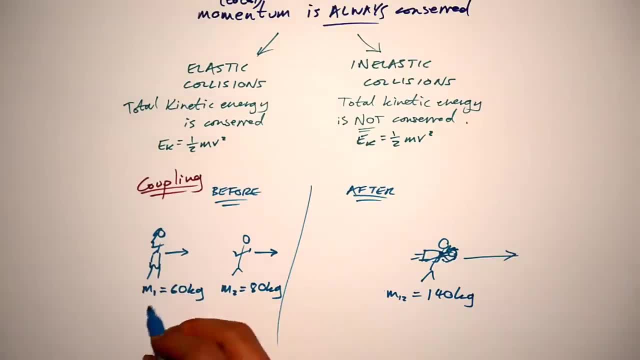 they're going off together. What do we know about the speeds? Well, we know that's from Souvat. when we have an initial speed before and a speed afterwards, generally we use u, so I'm going to put u1 and u2.. The girl to begin with has a speed of five meters per second. the guy only has a speed of. two meters per second. It alone cost s1 and some x now. but put u1 will do. If you put youot go现在 executive speed rhyme with a speed of 5 m per second. the guy only has a speed of two meters per second After that. 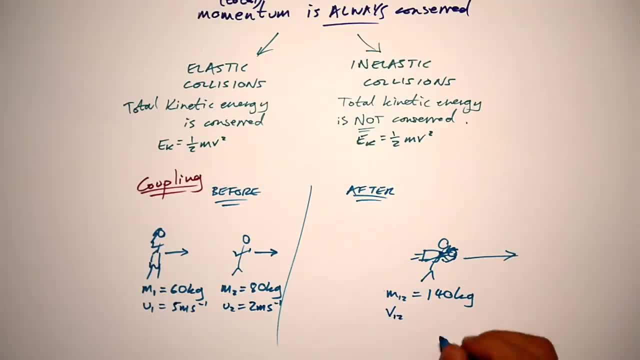 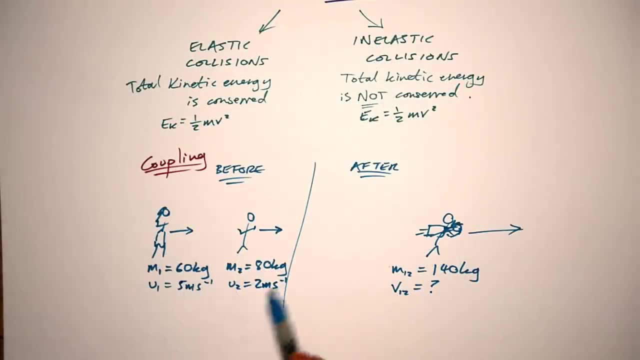 Afterwards. they've got a speed going off together, so I'm just going to put V12.. That's what I want to find out. So we need to come up with an equation for this. Now we know that the total momentum before equals the total momentum afterwards. 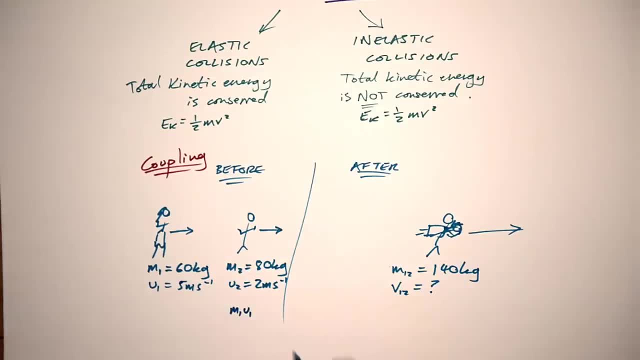 So we can say: M1U1,, that's the momentum of the girl, plus M2U2,, that's the momentum of the guy, equals M12,, that's the mass of both of them before times V12.. That's the velocity of them afterwards. 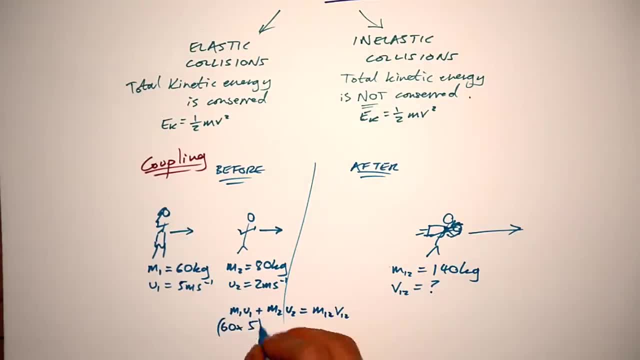 Pop some numbers in. We have 60 times 5, brackets. that plus 80 times 2, equals 140. lots of V. I'm just going to call that V. I can't be bothered to call it V12.. All you have to do then is rearrange it to find V. 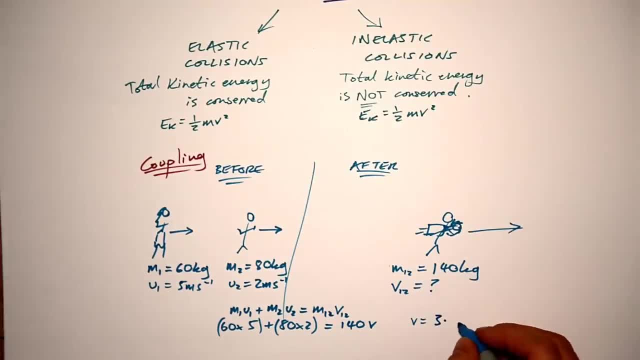 And we end up with a speed of 3.29 metres per second. All we did was figure out how to represent their momentums, their momenta before M and U. M and U, That's the total momentum before the collision. 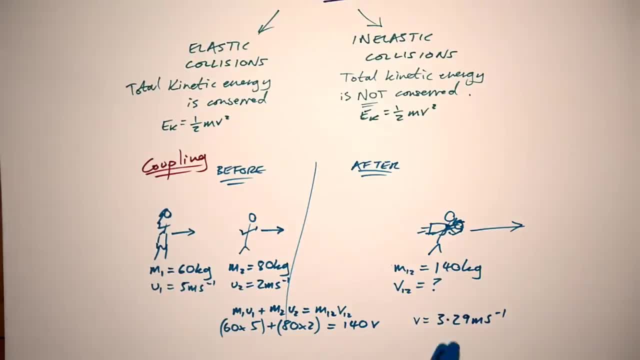 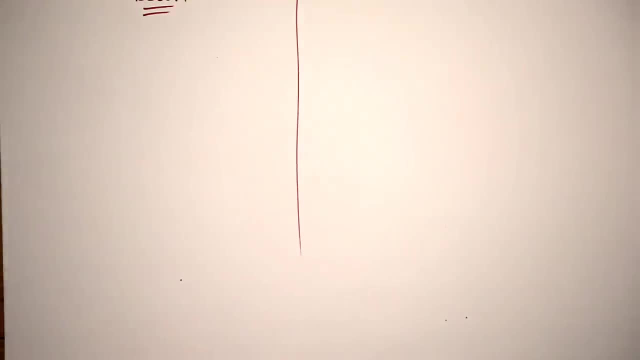 This is the total momentum after the collision. Make an equation, rearrange it and find the unknown. So that's coupling. Let's have a go at another one: Recall, say from a gun, like we were talking about earlier. We have before and we have after. 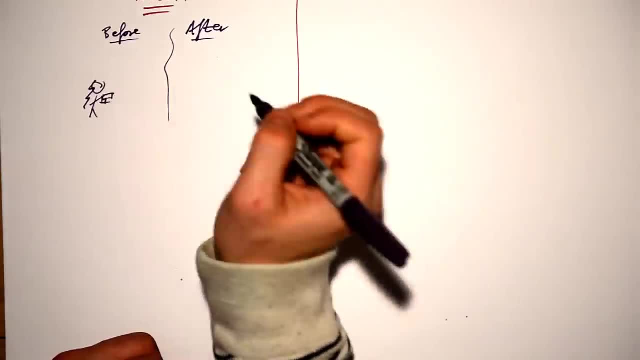 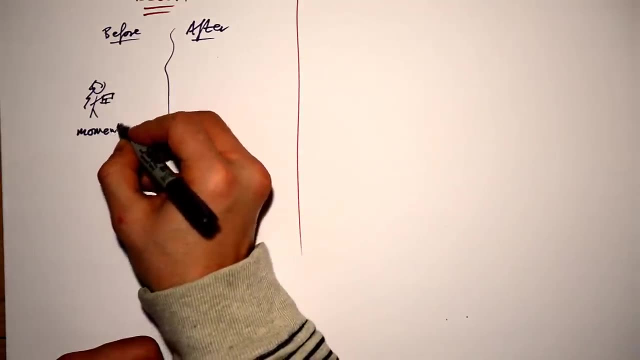 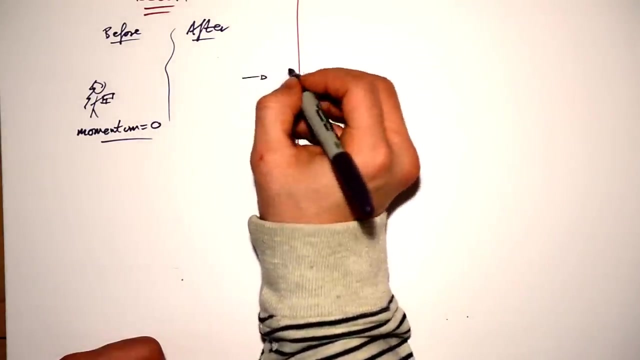 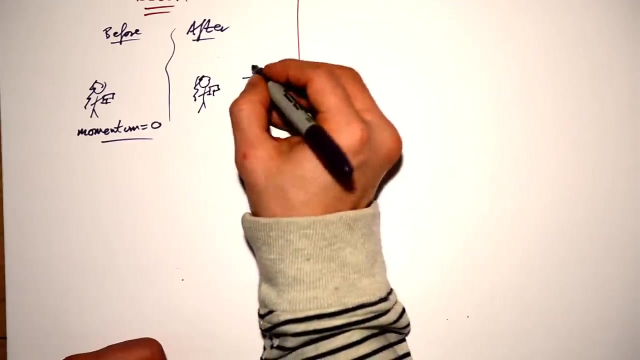 Before we have somebody with a gun and nothing's moving. How much momentum do we have Zero. We have no momentum Afterwards. the bullet's gone off in this direction And the shooter and the gun are obviously going to go backwards because of the recall. 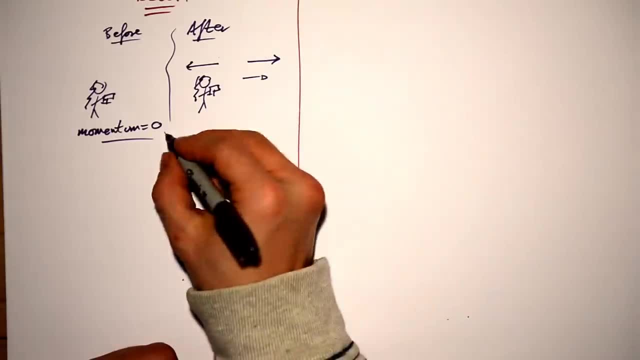 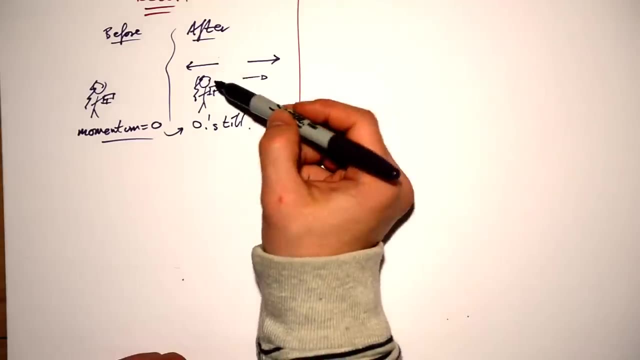 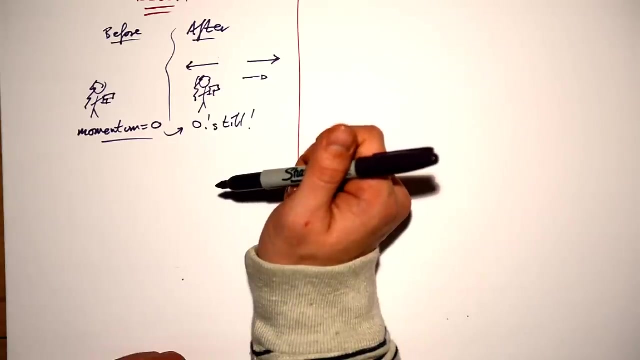 How much momentum should we have afterwards as well? Total momentum: Zero, Zero still. That must mean that the momentum of the bullet plus the momentum of the shooter and the gun must add up to zero. Does that make sense? Yes, because we know that the velocity of the bullet is positive. 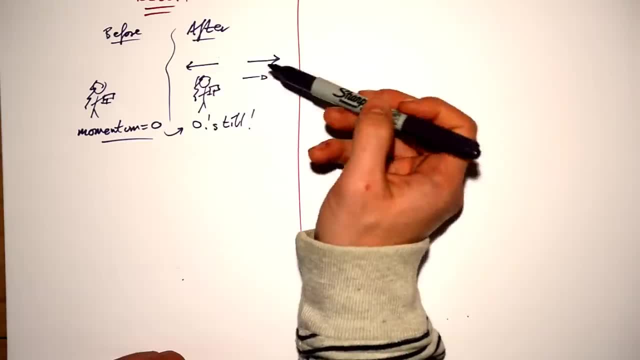 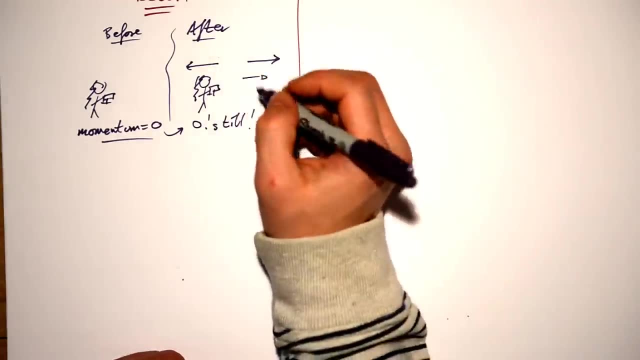 the velocity of the shooter and the gun is negative. So adding up momentum plus a negative momentum, they should cancel each other out and they add up to zero. So all I have to say is we have a mass here of the gun. 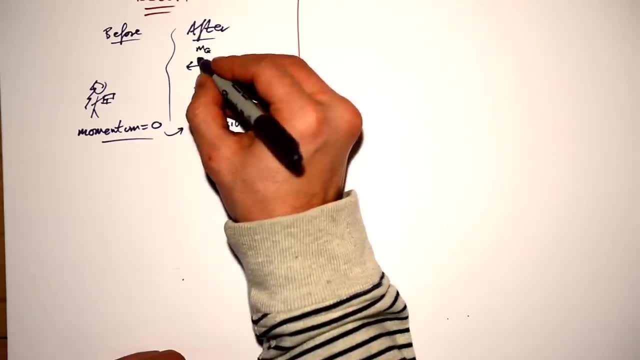 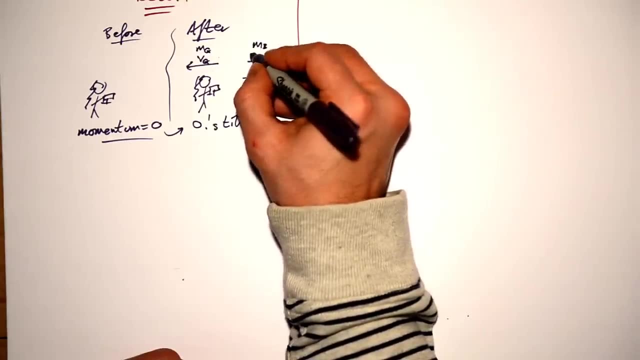 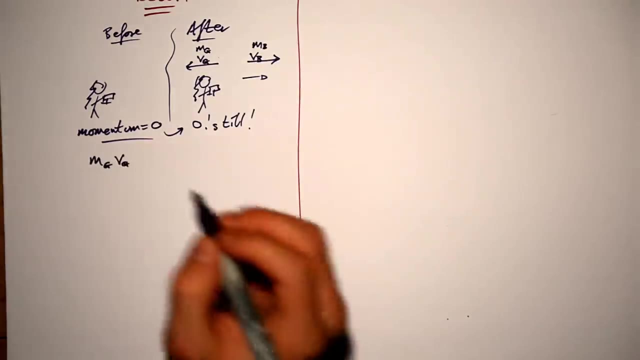 I'm going to call that mg, and we have the velocity of the gun as well, and the shooter as well, obviously, and we have the mass of the bullet, mb, and the velocity of the bullet as well, Making an equation. for this we just say mg, vg. 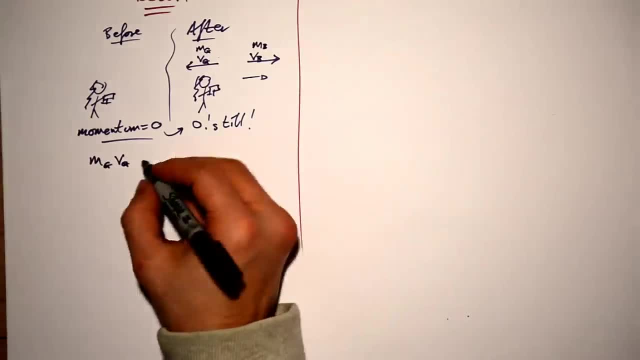 that's the momentum of the shooter and the gun plus the momentum of the bullet, plus the momentum of the gun plus the momentum of the bullet equals zero. Now you've got to be careful with the whole negative velocity thing. There is a bit of a shortcut that I like to use. 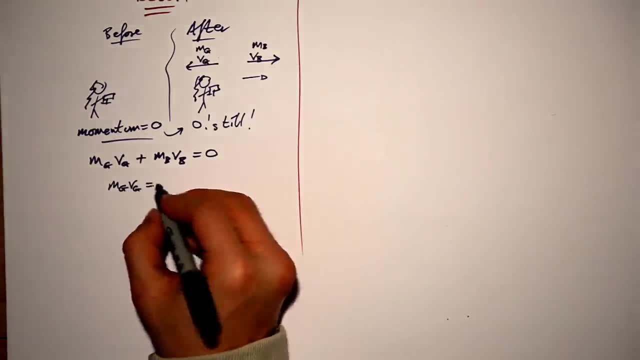 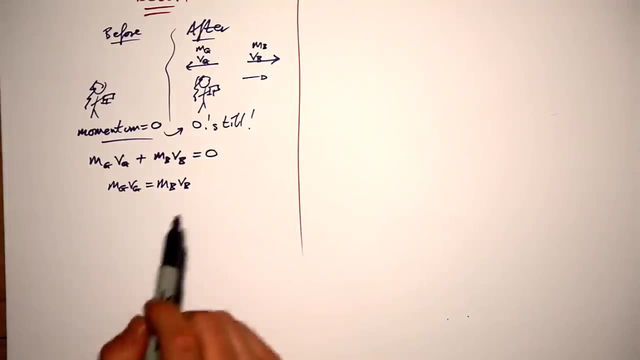 I just like saying: well, I know the momentum of the bullet is going to be the same as the momentum of the gun and the shooter afterwards. This isn't quite true because, of course, one of these is going to be negative compared to the other velocity. 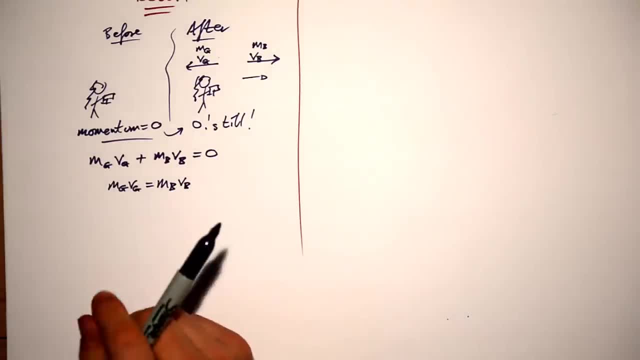 But so long as you remember that one of them is going one way and one of them is going the other way, let's be honest. you can remember that, then you should be fine. So let's use the same mass of the bullet. 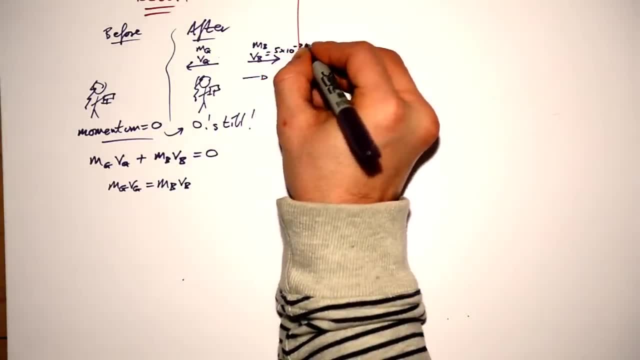 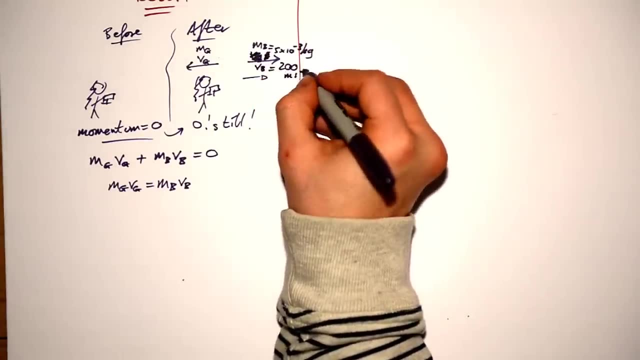 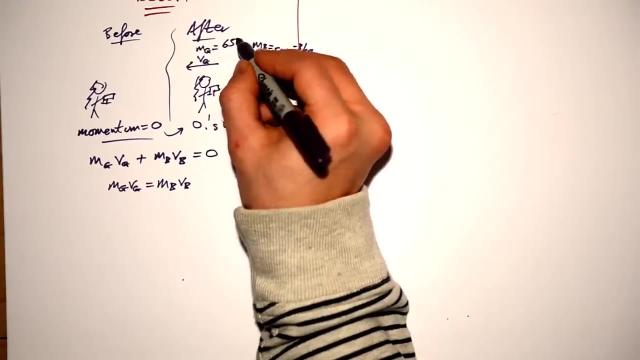 I'm going to say that that is 5 times 10 to the minus 3 kilograms, and the speed of the bullet again is 200 meters per second, Now, although the mass of the gun and the girl is 65 kilograms. 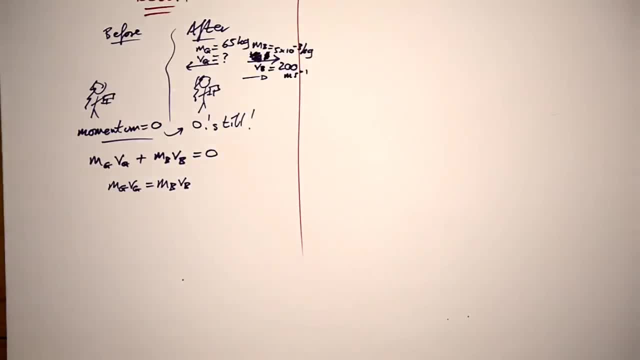 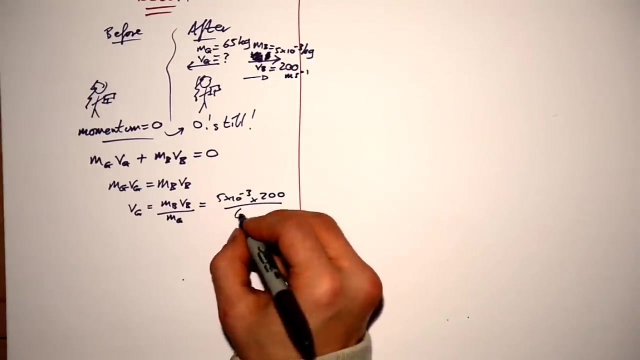 so I want to find out the recoil speed of them going backwards. What I want to do is rearrange this to find that speed, that velocity, And we end up with 5 times 10 to the minus 3 times 200 divided by 65.. 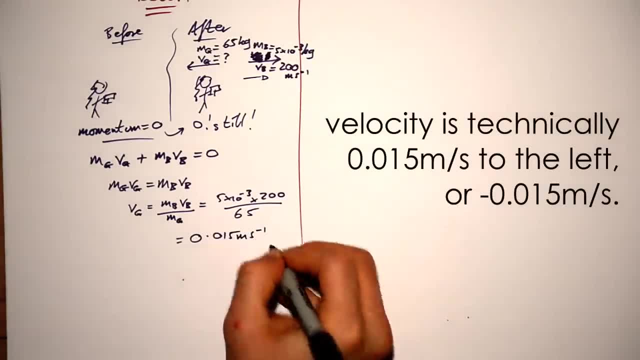 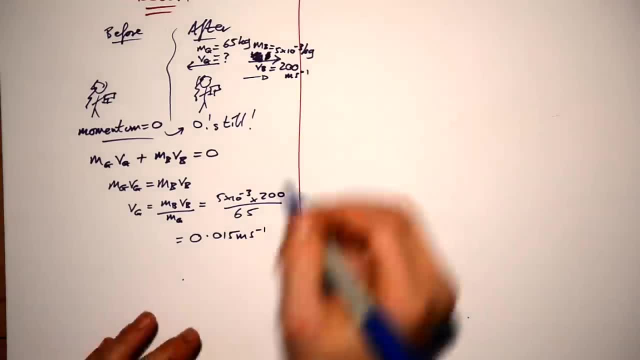 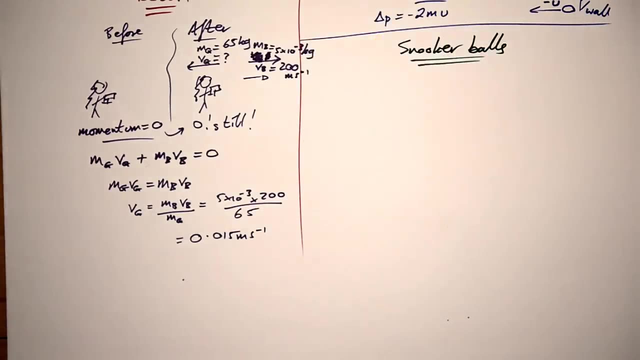 That gives me 0.015 meters per second, Not going back very fast. It is only a small bullet after all, So that's recoil. We also have rebound. Now, when Stuka balls hit each other, they have two options. 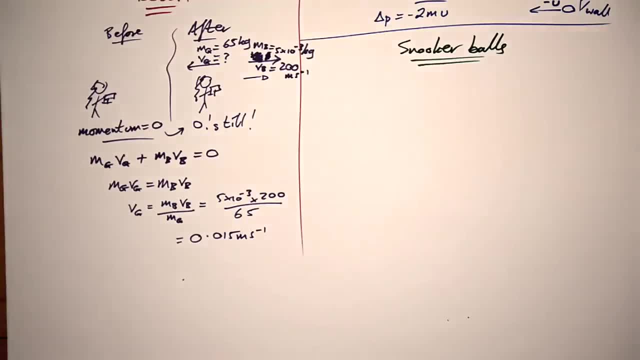 Well, three options really. The cue ball can hit the other ball and it can just stop dead. The cue ball can carry on going if you put some topspin on it, or it could come backwards if you put some backspin on it as well. 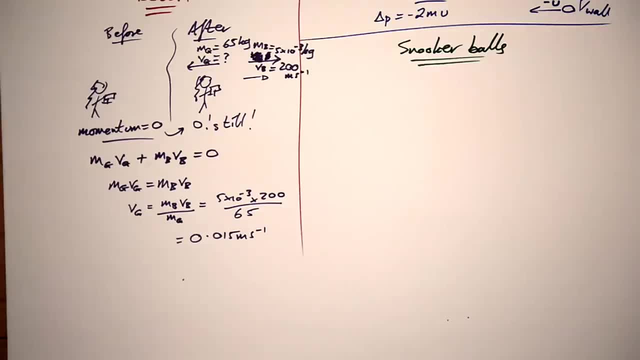 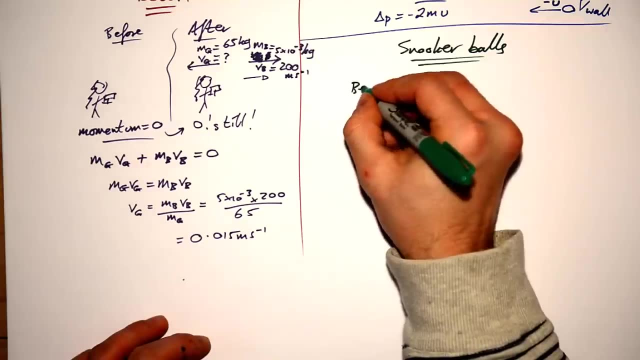 The problem with those is that they do affect whether the collisions are elastic or inelastic. But let's not worry about that for now. Let's just worry about the actual- uh, momentum side of things. So we have before and we have after. 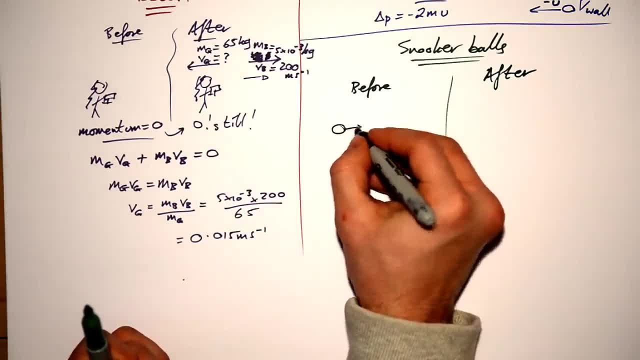 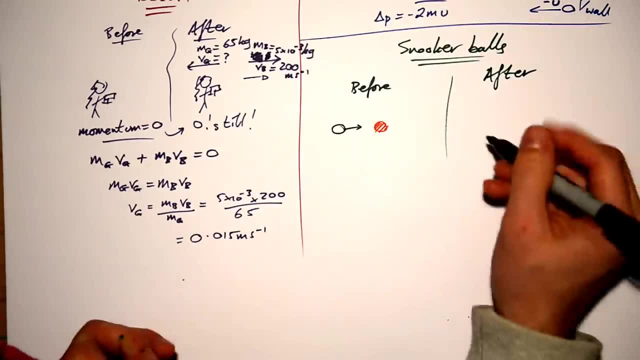 So we have our cue ball coming in and that's going to hit the red, which is staying still at the minute. Afterwards, let's say that our cue ball goes backwards. we put some backspin on it and the cue ball's going up in that direction. 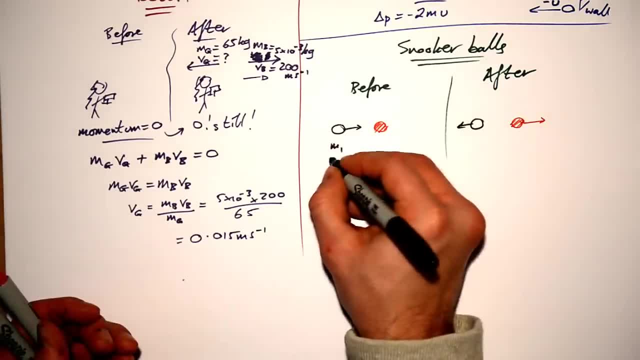 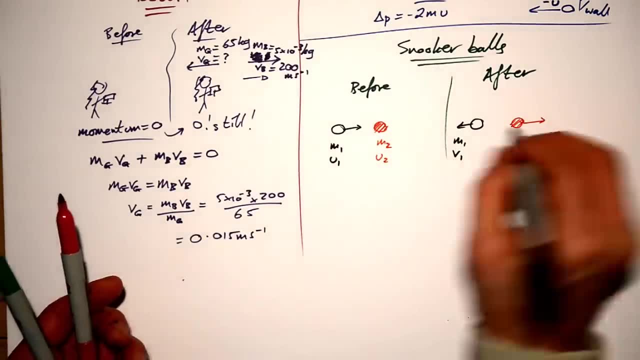 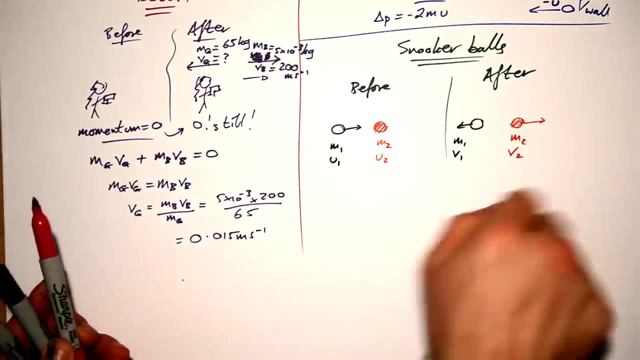 hopefully going into the pocket Again. we have M1, U1, M2, U2, M1, V1, and we have M2, V2.. Now, no matter what is going on with this whole situation, we can say that M1, U1,. 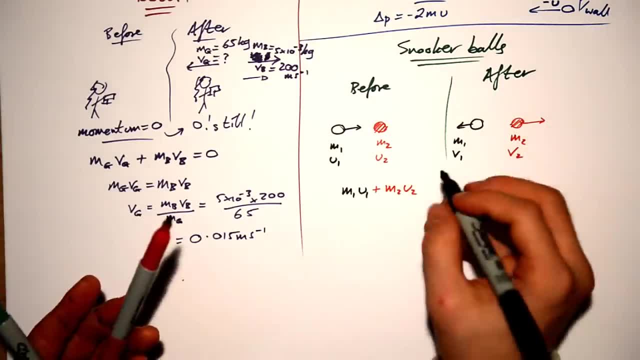 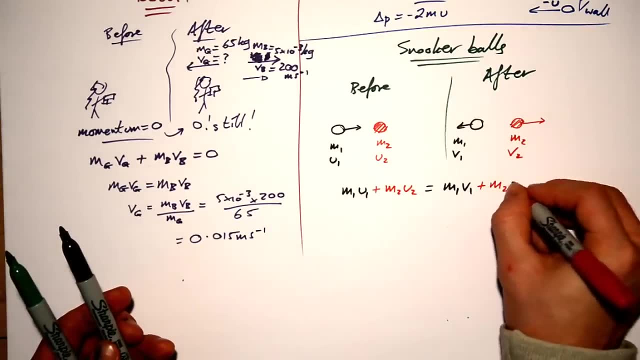 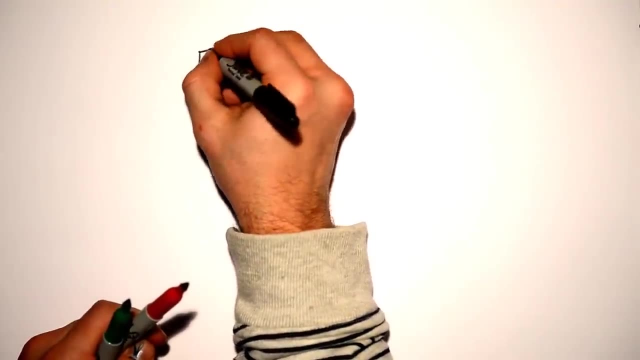 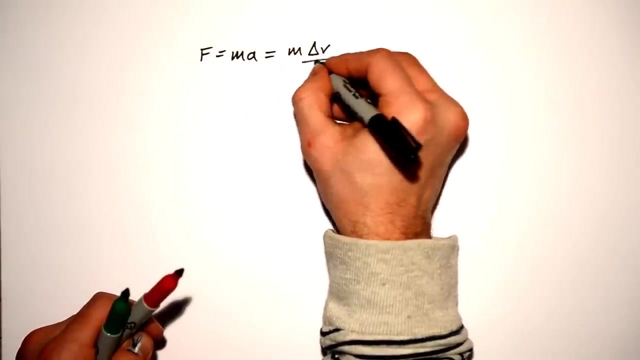 M2, U2 equals M1, V1 plus M2, V2.. Let's go back to Newton's second law, That is, F equals MA. What is acceleration? Well, it's change in speed over time. So I can put M delta V over T. 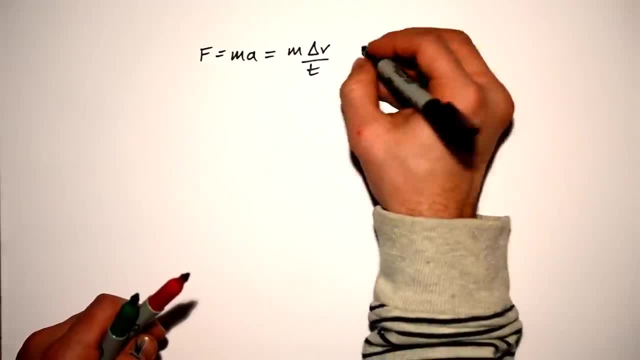 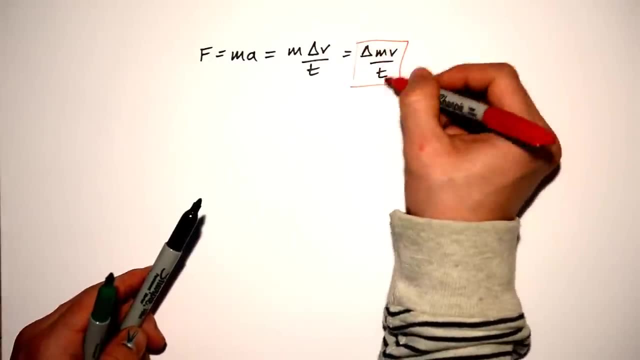 Actually, it doesn't have to be V, that's changing. It could be M as well, So I'm going to put a delta in front of both of those two things together. This, if you will, is the more accurate version of Newton's second law. 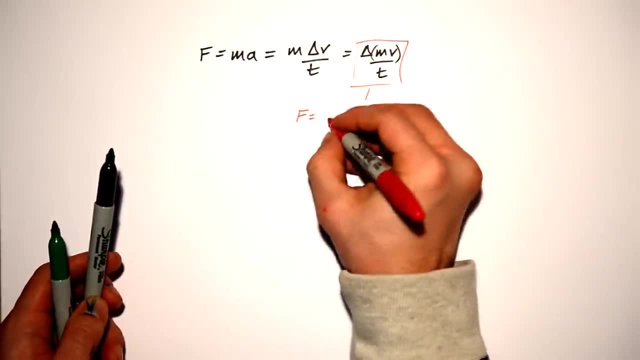 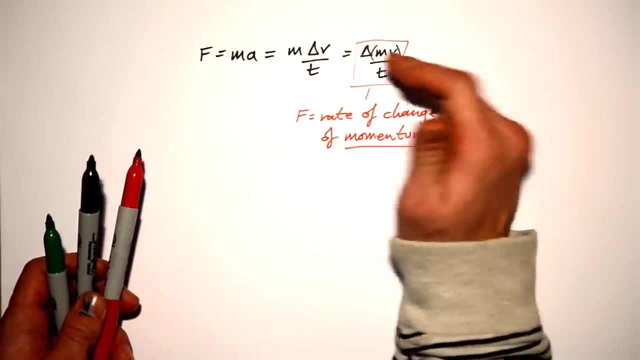 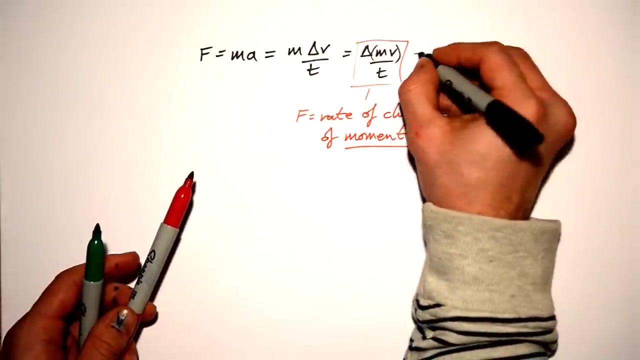 This is saying that force is equals to the rate of change of momentum, MV momentum divided by T: delta, change in momentum over time. Anything divided by T is the rate of the change of that something. I could actually write this as then. 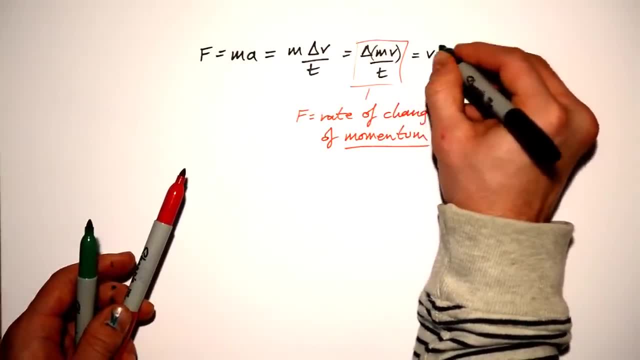 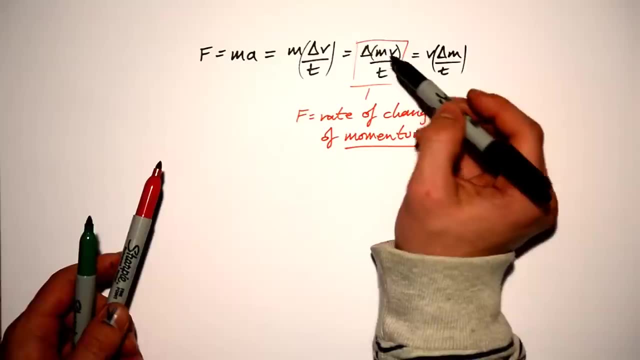 V. delta, REM over T Same thing just depends on what's changing. Is it the mass that's changing or the velocity? Generally, you will never have a situation where both the mass and the velocity are changing at the same time. It'll either be the velocity changing. 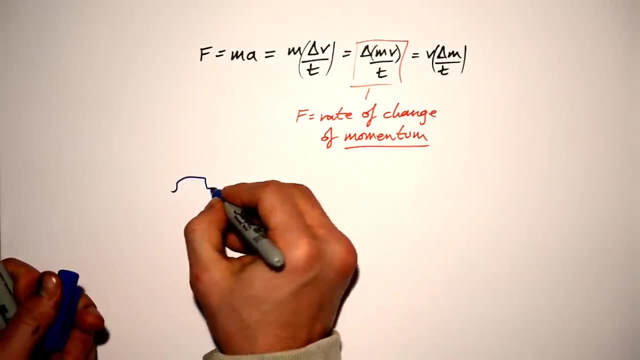 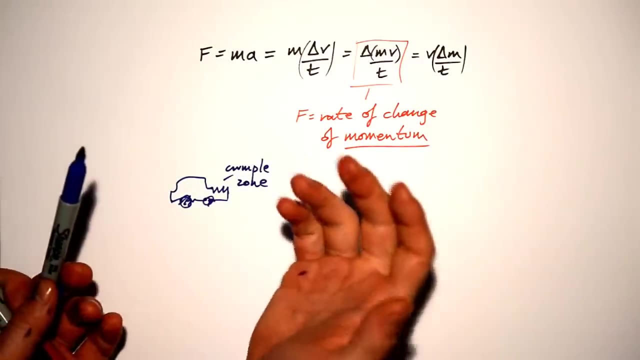 or the mass is changing. So on cars you have something called crumple zones. If you're in a car crash, your momentum is going to come down to zero every single time. That's not going to change whether you have a crumple zone or not. 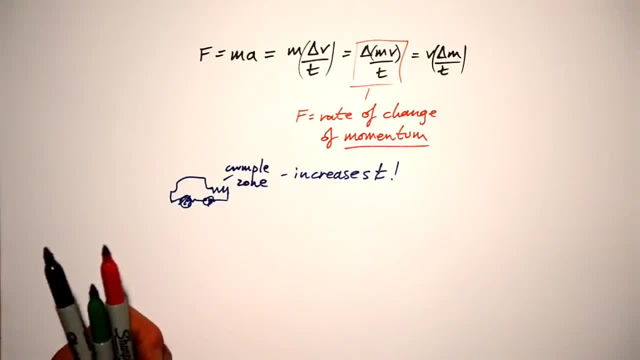 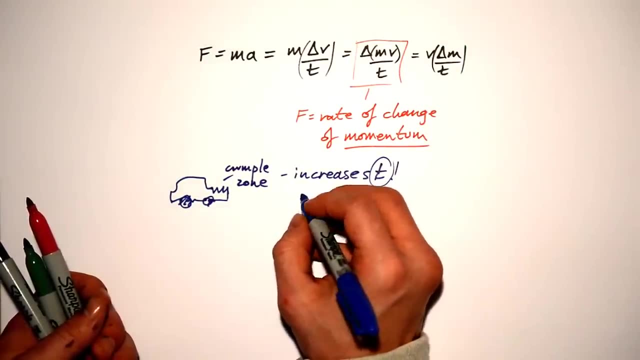 But what does a crumple zone do? It increases the time of the collision. What does that mean? If you increase T, that means that the rate of change of momentum is lower. So therefore F is lower If you get fired out of a cannon. 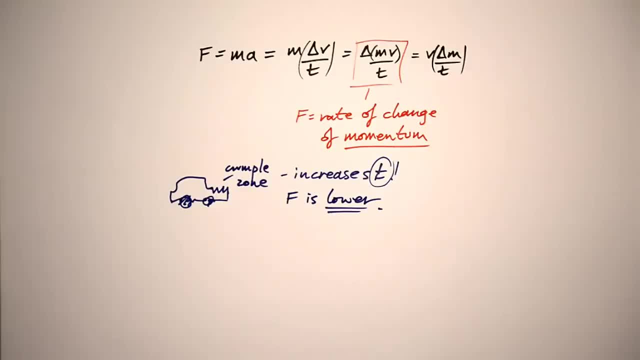 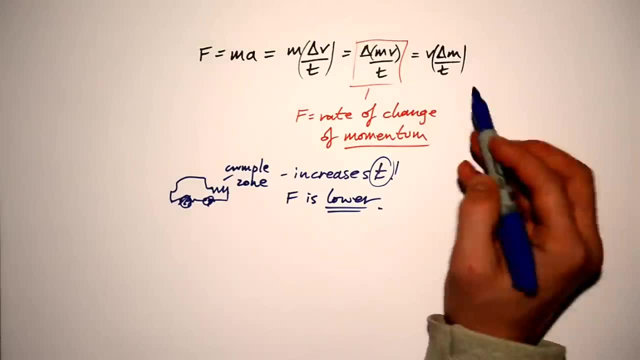 then you've got a choice of hitting a wall or hitting a nice big net. Your momentum is going to come down to zero either way. Which one's better? Of course the net is because the time for that collision is going to be longer. 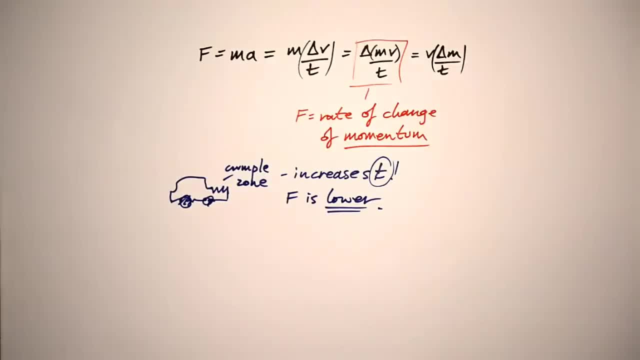 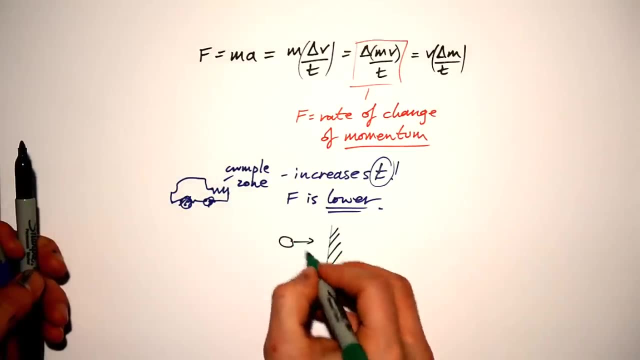 so the force you feel is less, and so you'll probably survive that. Let's very quickly look at our ball. that's hitting a wall again, Like so, and we have it going in here and we have it coming out there. It's going in with U. 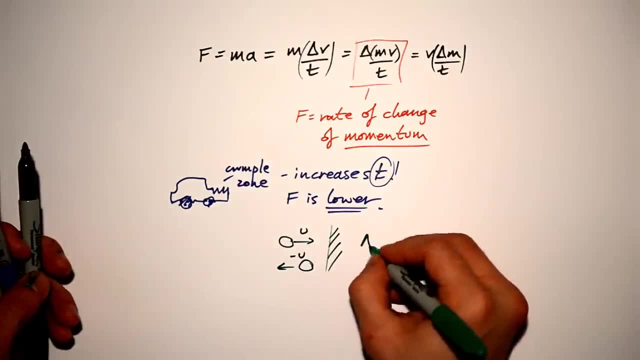 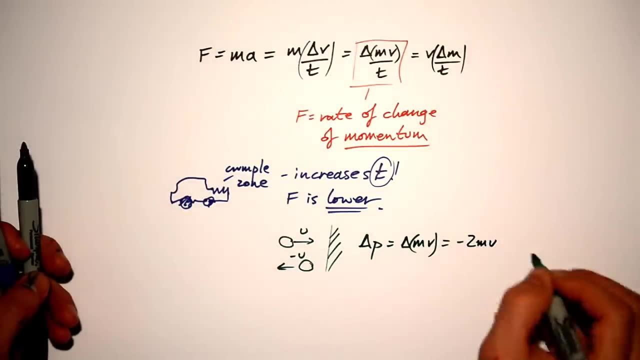 and it's coming out with minus U. We said that the change in momentum, I could say delta P, that's also delta MV. of course that's going to be minus 2 MU. So that means that the force exerted on this wall by this ball 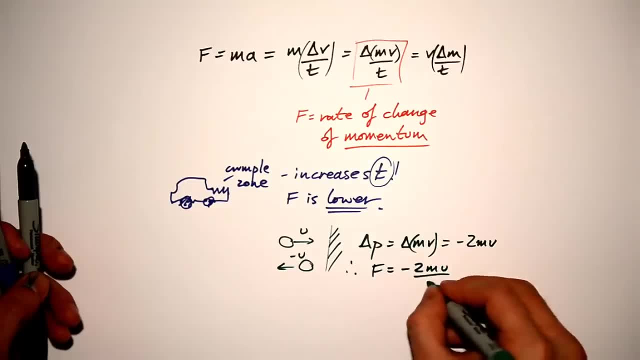 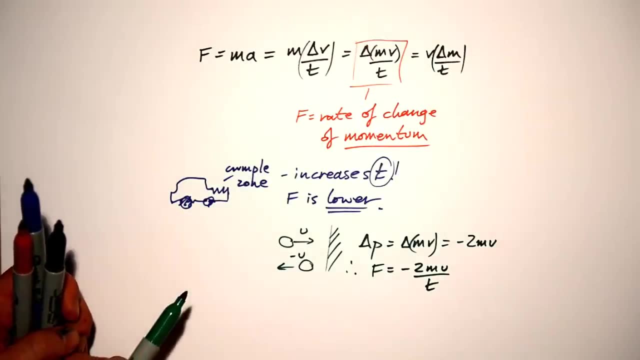 is going to be minus 2 MU over the collision time. That is how long it's in contact with the wall. The longer it's in contact- say it's a really deflated football- then it's not going to be exerting much of a force. 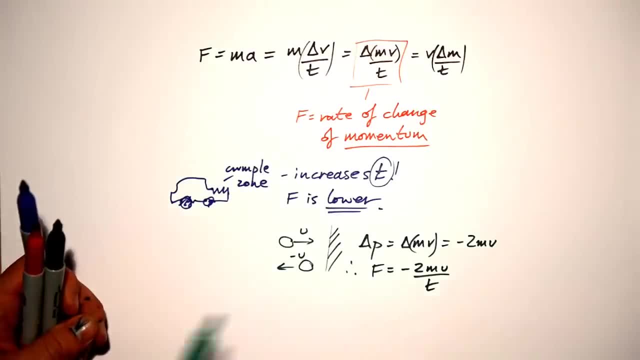 If that's a massive ball bearing, then the collision time is going to be very short. So that means T is small, the force is going to be quite big. Change in momentum is also known as impulse. So whenever you see impulse it just means a change in momentum. 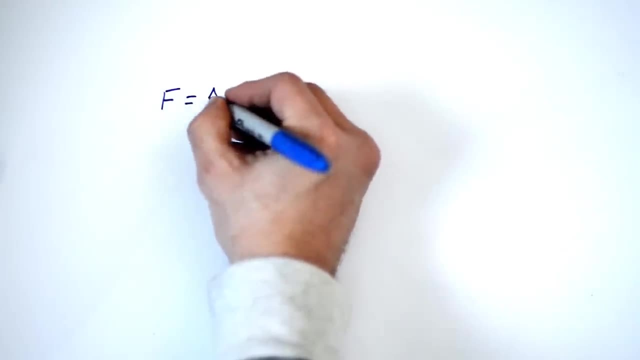 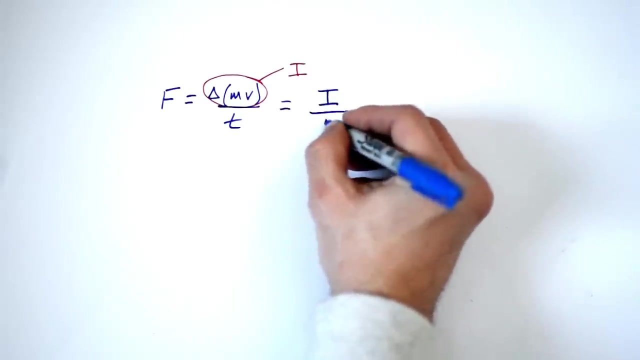 Same units. So if F equals change in momentum over time, there should be a delta before that. We call the T as well, but we leave that out And we said that this is impulse. given the letter I, then that means that force is equals to impulse. 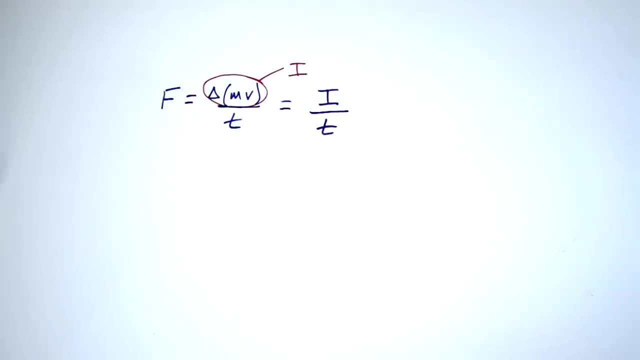 divided by time. Same thing, just that impulse is change in momentum. You might get given a graph. This will be a force-time graph. Now, whatever shape the graph makes, you know that the area under the graph is equals to the change in momentum or the impulse. 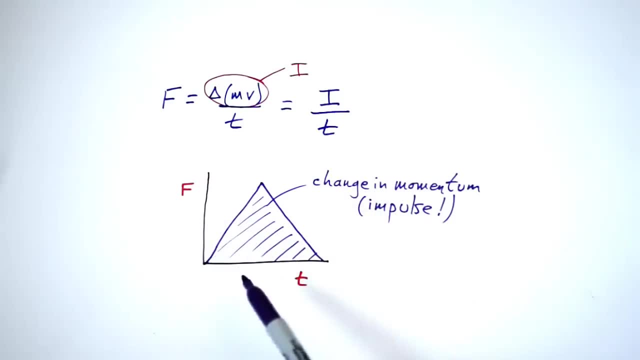 Just like if we have a speed-time graph and we find the area under the graph. we find distance. Here, if we have force and time, find the area under the graph and we find the impulse, the change in momentum, As per usual. 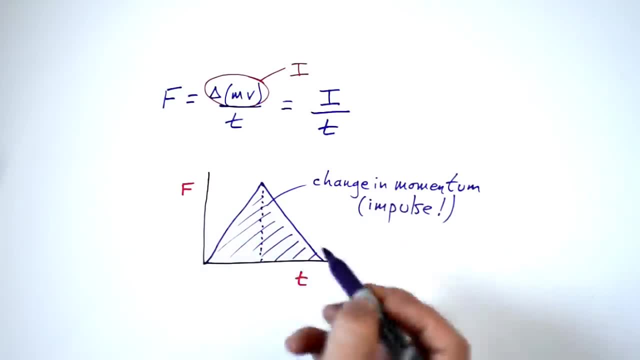 split it into rectangles and triangles. So I split this into two triangles: Base times height divided by two. Base times height divided by two. Add them all up and you find the change in momentum. Usually, whatever is experiencing, this change in momentum starts at rest. 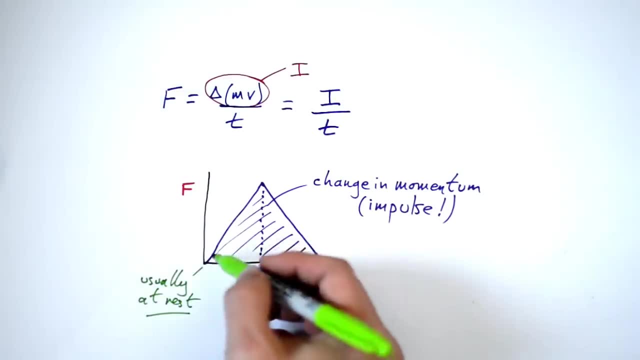 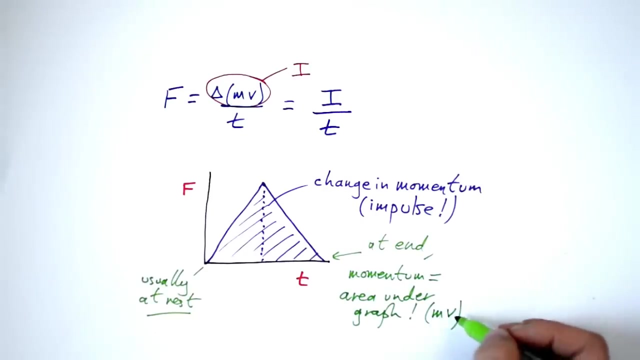 So that means no momentum at all. So by the end, the momentum that this object has is going to be the area under the graph, because it didn't have any to begin with. That's going to be equals to mv. Then if you're trying to find the velocity, 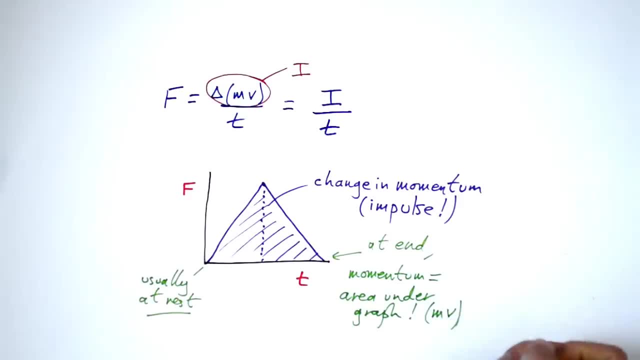 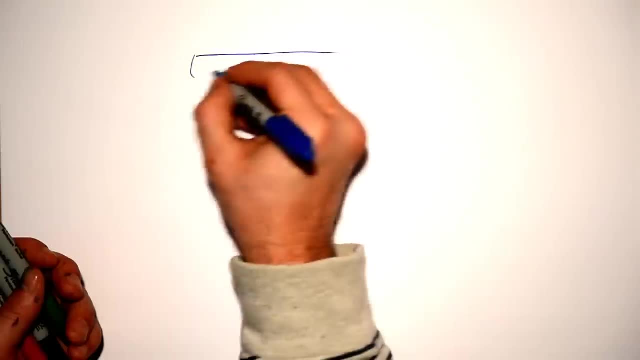 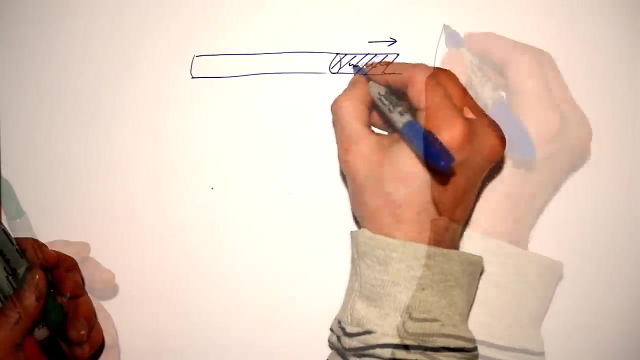 just divide the area under the graph by the mass and you find the speed. Now let's talk about one situation that confuses quite a few people. Let's talk about a hosepipe where we have water coming out. If this water then hits a wall, 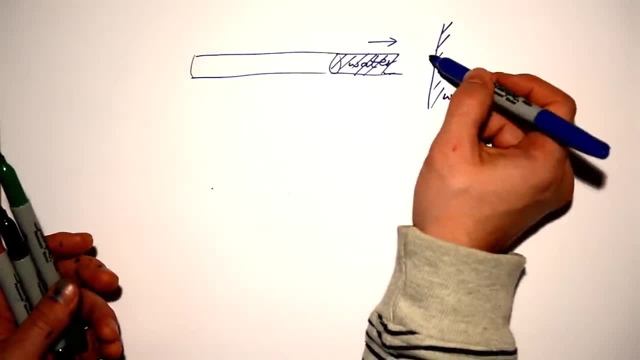 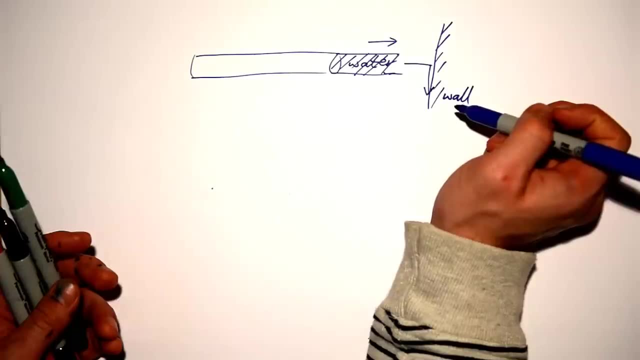 and it stops dead if it comes back, obviously we have a greater change in momentum than it's just momentum If it stops dead. we don't really have a collision time because there's a constant flow of water. So how on earth are we going to find out? 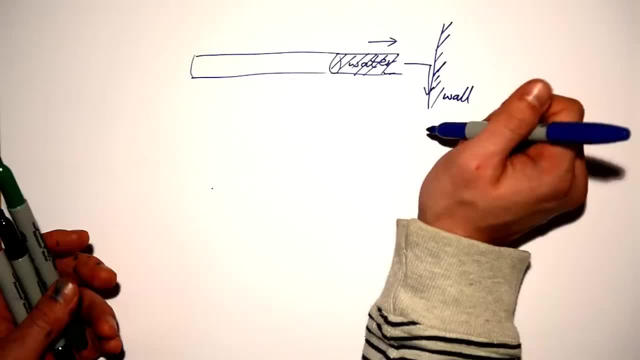 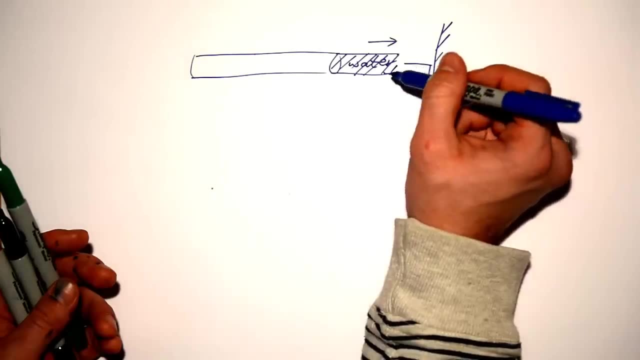 what the force is exerted on this wall, by this stream of water. By the way, it doesn't matter if there's a wall or not. If there isn't a wall, the question will say something like calculate the change in momentum every second. 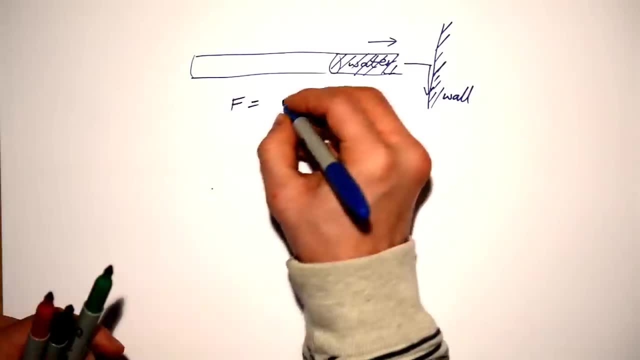 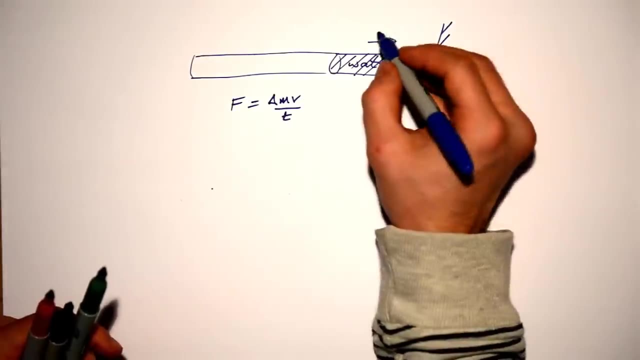 which just means effectively find the force. Let's write down our equation: F equals delta mv over t. Now then, if the water is flowing out of here at a constant rate, v, then obviously v isn't changing at all. So let's take v out of the equation. 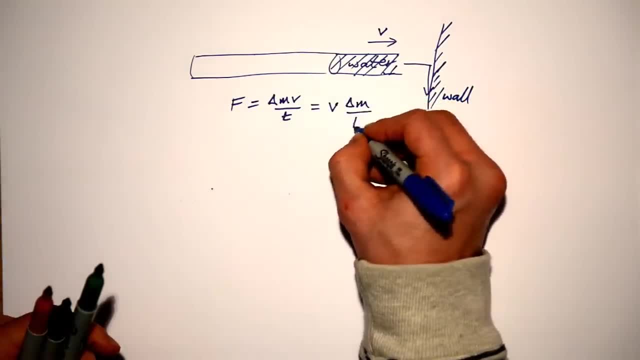 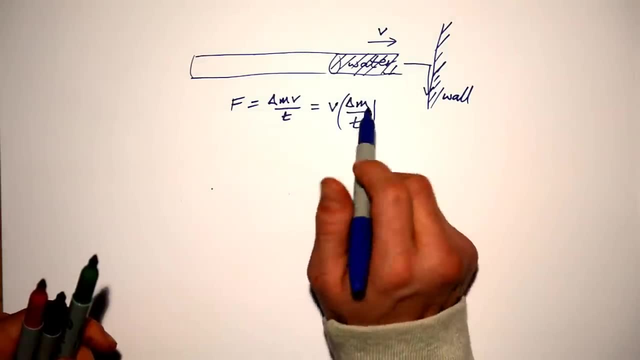 The equation there And instead we've got delta m divided by t there. This is true. The force exerted on the wall by the water, if it stops dead, is going to be the speed of the water times, the change in mass per second. 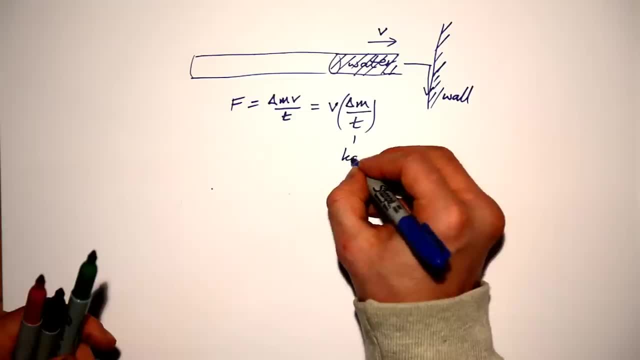 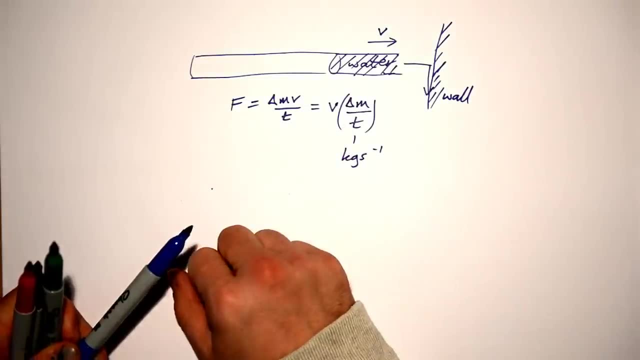 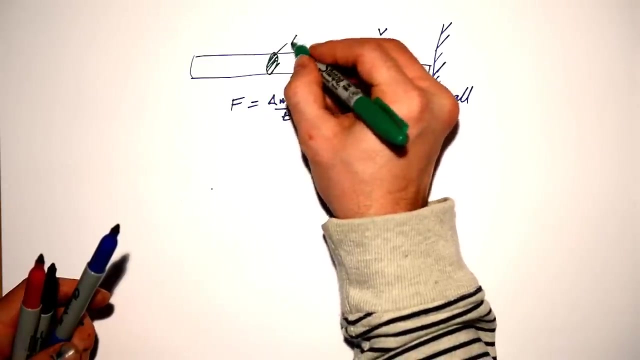 In other words, kilograms per second. This is one time where units are definitely your friends, because you will not get given an equation for this, But we're going to derive one now. Now I can tell you that this hose pipe has a cross-sectional area A. 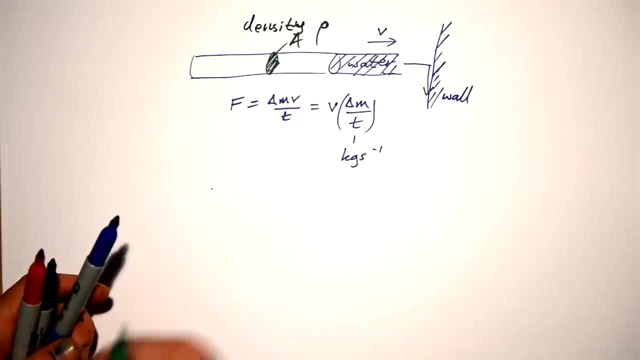 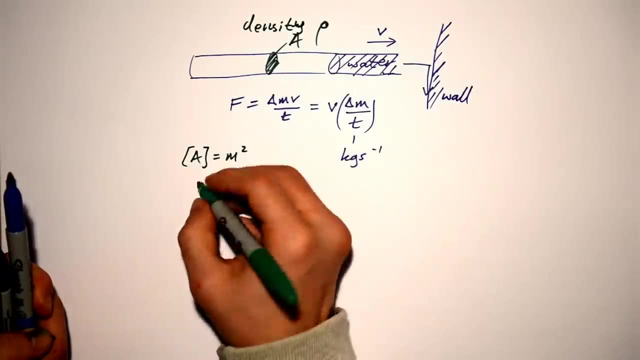 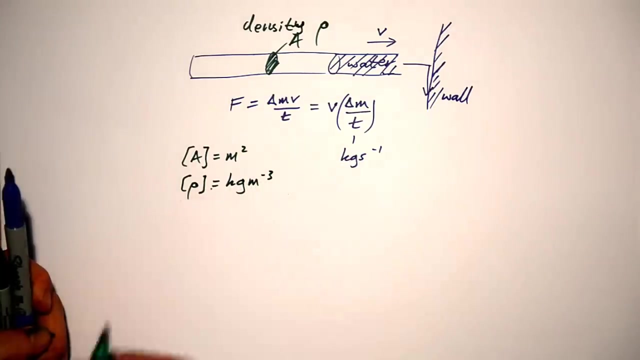 and the water has a density: rho. That's not a p, that's a rho. It's a p without a little e. Now, area has the units meters squared. Rho has the units kilograms per meter cubed. Now we want to get. 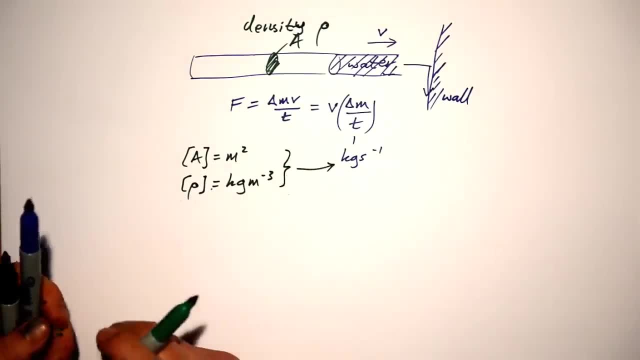 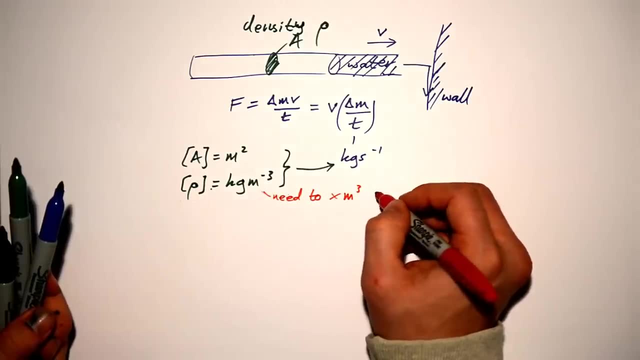 from these two to kilograms per second, And we need to times by meters cubed, because of course there's no meters cubed in here at all. There's no meters at all. And we need to times by s to the minus one as well. 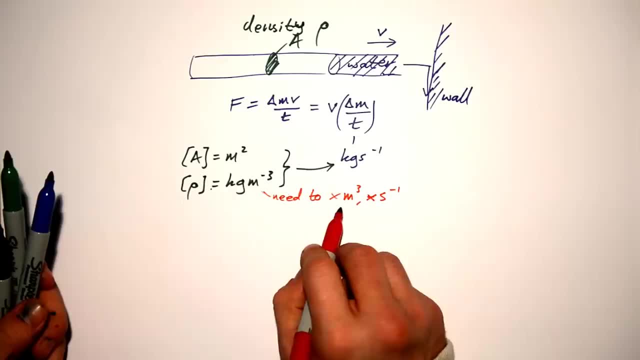 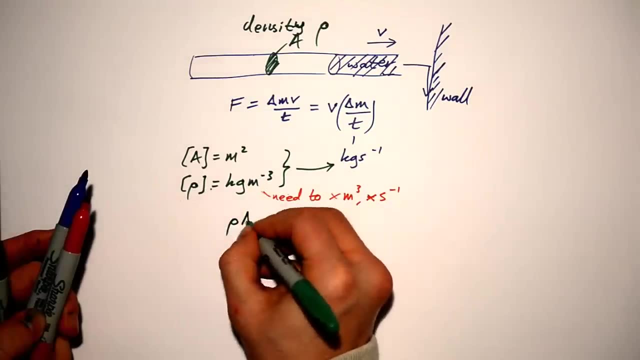 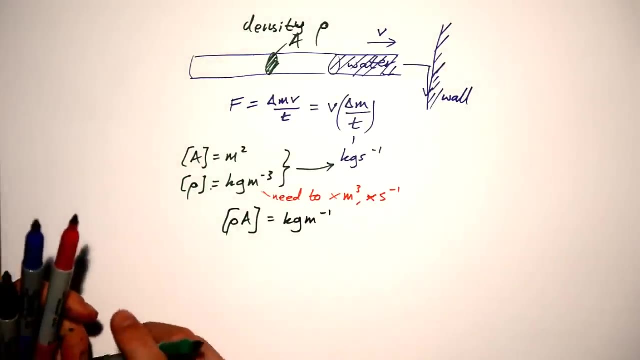 because we have that. So where are we going to get our meters cubed from? Well, look, we have meters squared up here. So let's do A times rho, or rho times A. That gives us kilograms per meter. That doesn't really tell us much. 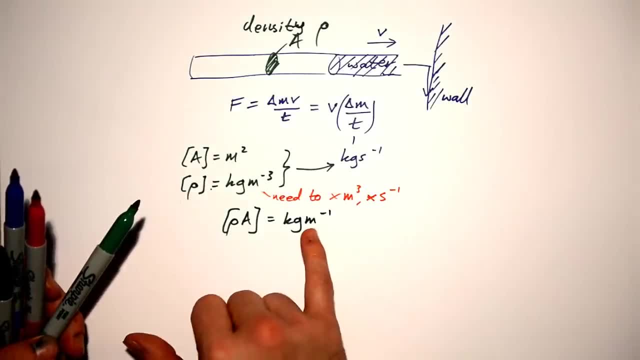 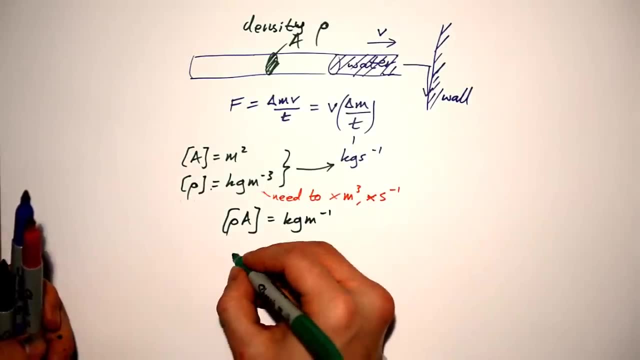 at the minute. We need something else. We need to get rid of this. meters to the minus one, And we need to add our seconds to the minus one in there as well. What do we do? We times by the velocity. Rho A v. 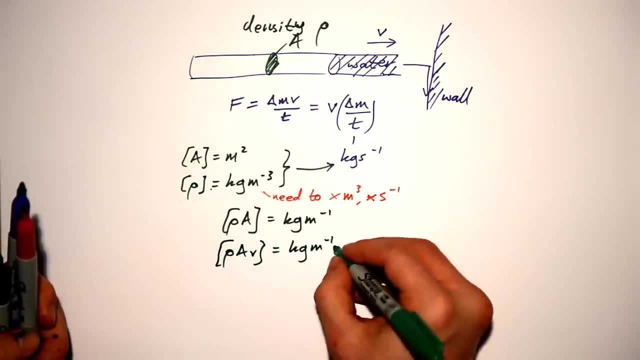 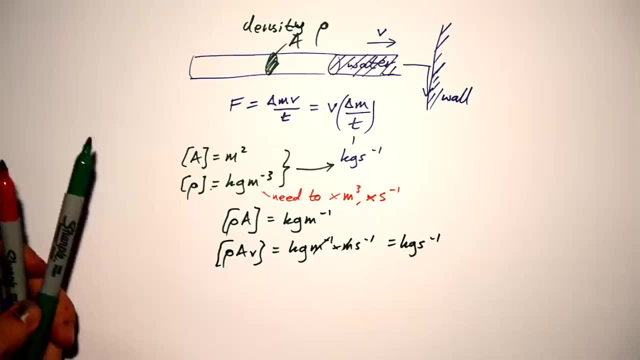 gives us kilograms per meter times meters per second. Those cancel and we get kilograms per second. So the change in mass per second for a fluid coming out of a pipe of cross-sectional area A is rho A v. To turn that into our force there. 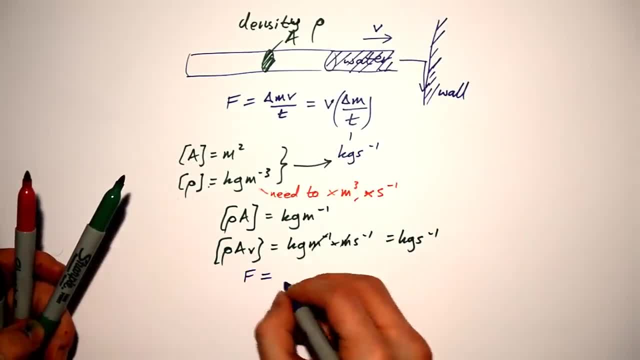 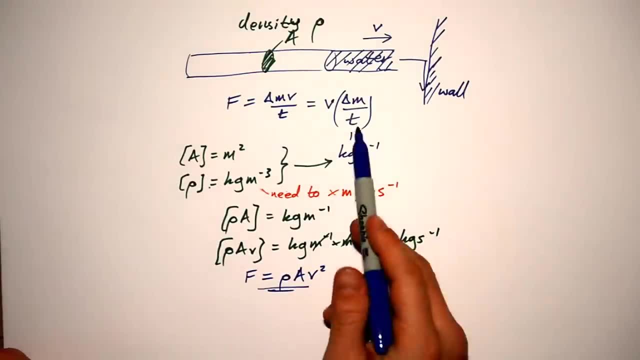 all we have to do, of course, is times by velocity once more, So we end up with rho A v squared. This is a bespoke equation with respect to what we're given in the question, But quite often you might not be given density, and so you'll have to. 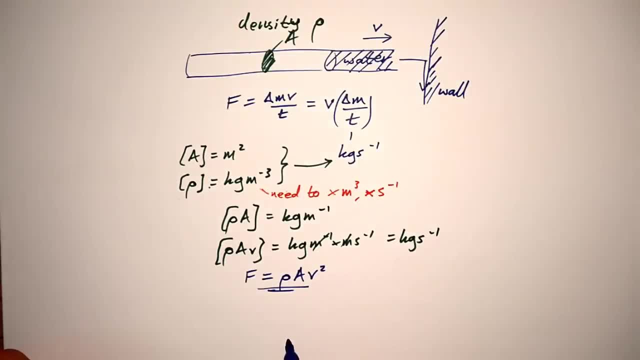 work through this whole process of figuring out what units you actually need to end up with in order to find out the force. Make sure you write down the units of all the information that you're given in the question and I guarantee that it will become clear. 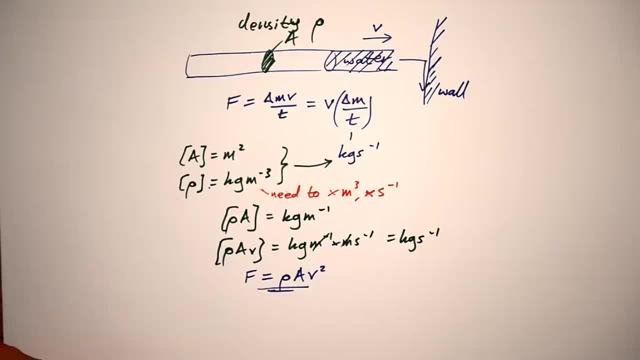 So I hope that helps. If you have any questions, please leave them in the comments below and I'll try and answer them as soon as I can See you next time. 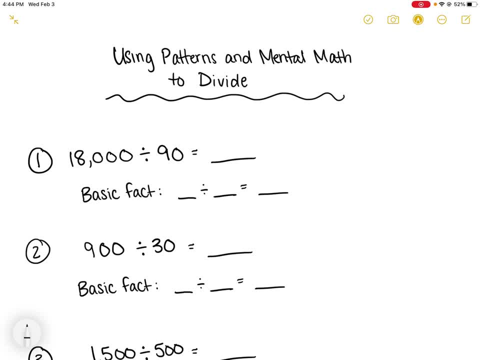 Today we will be using patterns and mental math to learn how to divide large numbers. So let's jump in and start with number one. For number one, we have 18,000 divided by 90. So the first thing you're going to do when you have a big problem like this is look for the 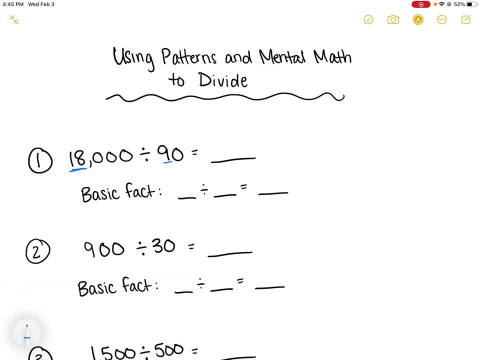 basic fact. So here we have 18 divided by 9.. 18 divided by 9, we know, gives us 2.. So that's the first part of our answer. After that we have to ask ourselves how many zeros is in my answer? 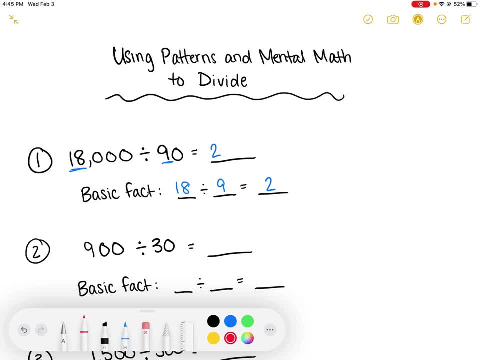 And to find out how many zeros are in your answer you'd look at the zeros in the problem. So for 90, we have one zero And 18,000, we have three zeros. So the zeros will cancel each other out. So since 90 has one zero, that means I can cancel out one zero in 18,000.. Now to answer the. 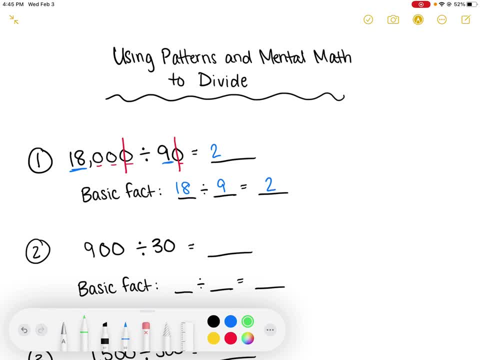 question of how many zeros are in our answer. we just look to see how many zeros are left over after the first part of our answer. So let's look at the first part of our answer. So we have two zeros left over. So that means there will be two zeros in my answer. So that means that.